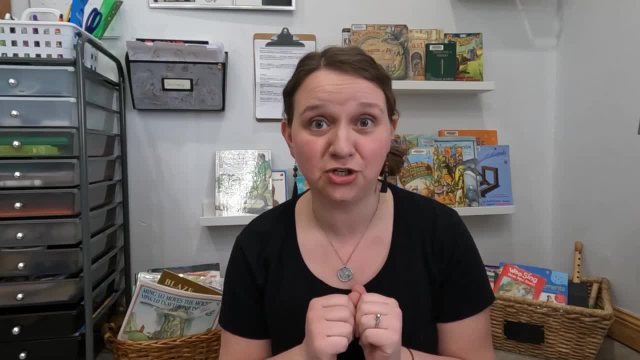 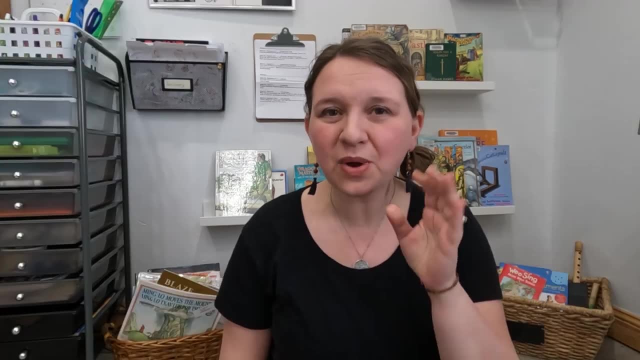 and I would recommend you checking that one out for next year. The second curriculum you shouldn't buy this year is anything that's going to stress out your homeschool budget, And I hope you have a homeschool budget and aren't just taking out of your family's budget. We need to separate those. 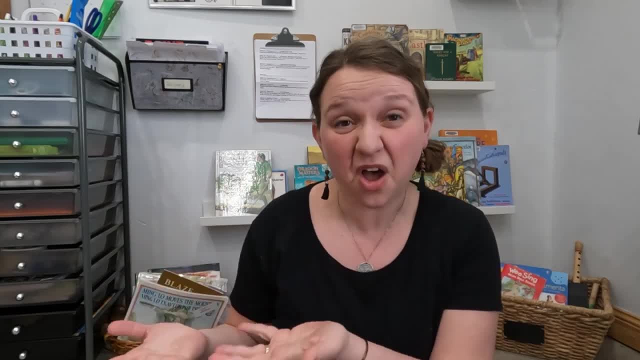 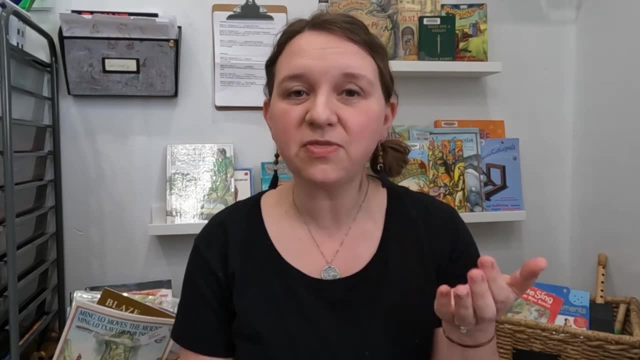 two, so that you don't have guilt and you know what the limits are for your homeschool. Now there are so many things that you shouldn't buy this year that are going to stress out your homeschool budget. There are so many curriculums out there, even for free, So if something doesn't fit in your budget, 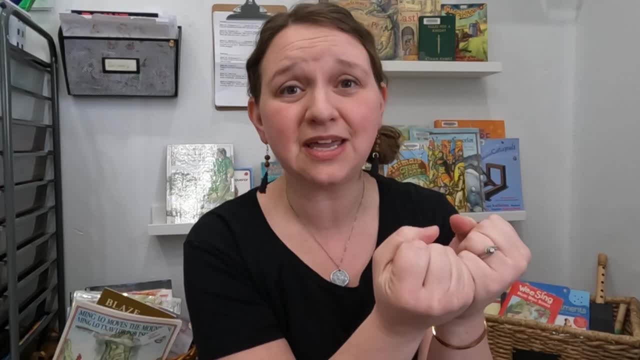 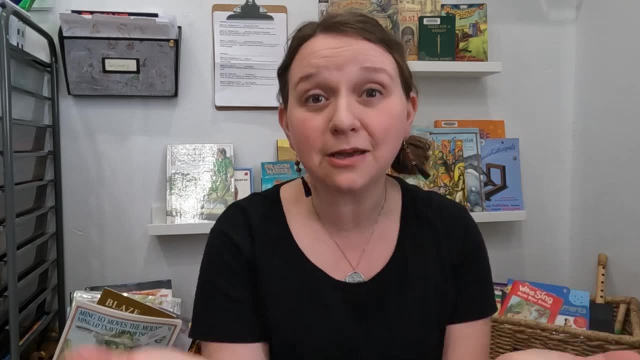 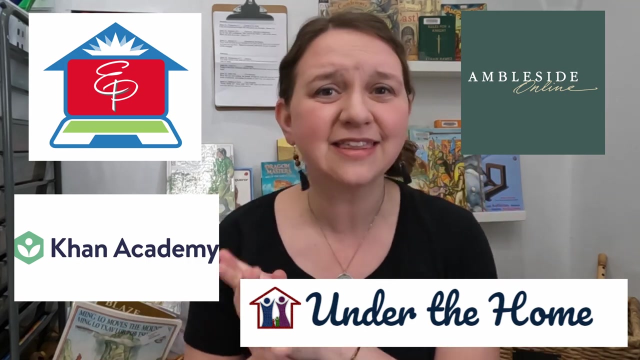 even if it looks like the perfect thing, don't do it If it's going to cause stress or division in your house or cause you to need to work extra to be able to pay for something like that. There are so many free options easy peasy under the home or under the house, something like that. 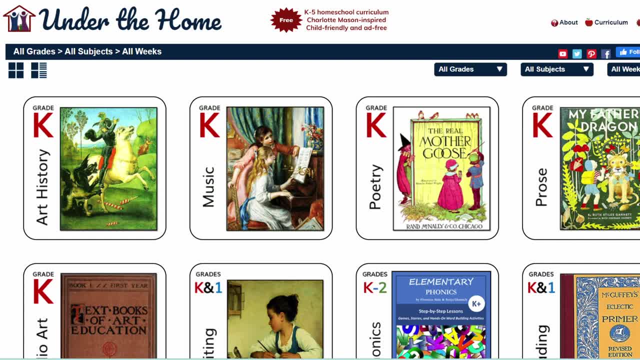 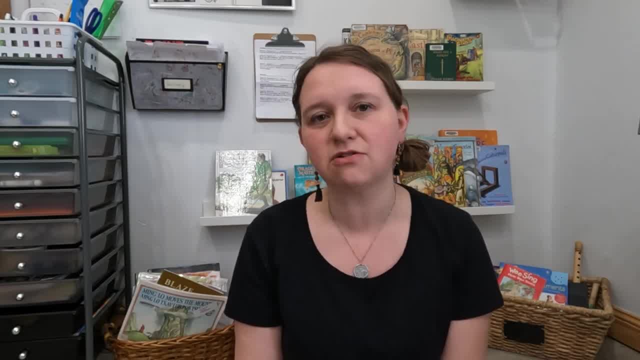 And they offer so many free curriculums, especially language arts, in there that you can be utilized for your homeschool budget. So if you're looking for something that doesn't fit in your budget, there's just so many options. It's not worth stressing out your family budget extra Now. 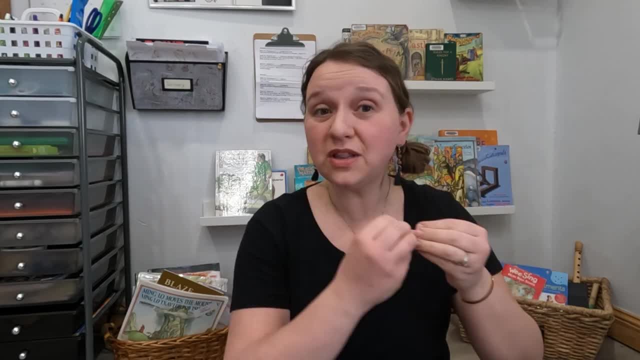 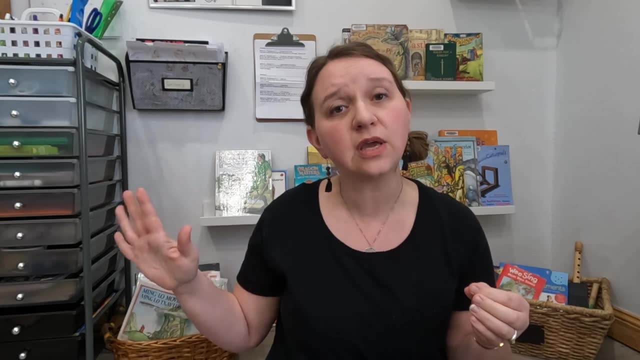 if there is one that you have really loved and you really want to make it work so that you can keep using it in your homeschool, then maybe just take a different curriculum and find a free way for it so that it frees up some of your money to be able to pay for that. There are options here. 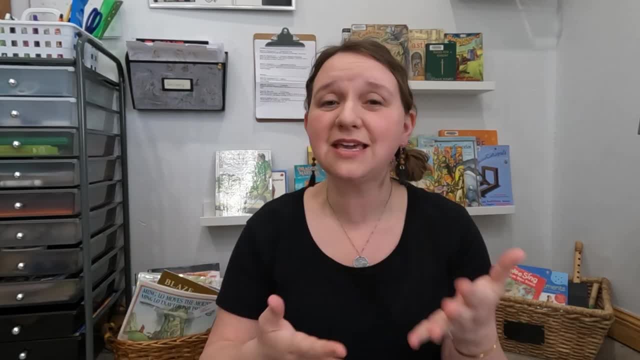 We homeschool because of flexibility and being able to make things work for our house, So don't feel like you have to spend a certain amount of money for that. If you're looking for something that doesn't fit in your budget, then maybe just take a different curriculum and find a free way for it. 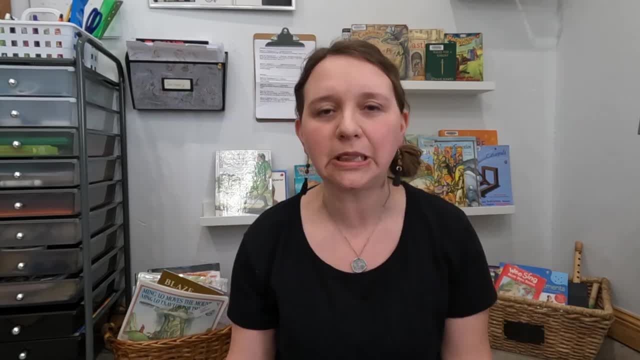 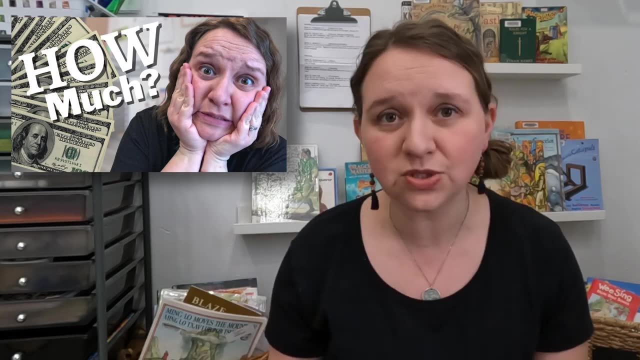 money for the perfect curriculum. There is no such thing as a perfect curriculum, and there are lots of options out there. Make sure to check out this video here that talks about the different price points of homeschooling curriculums, all the way from box curriculums that are $1,000 to free. So 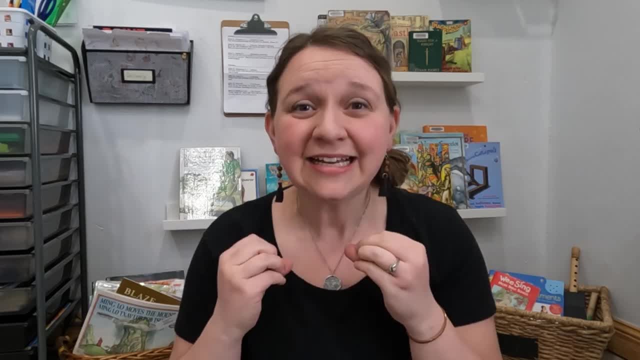 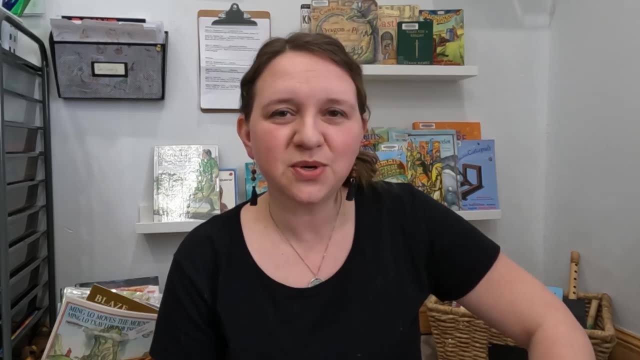 hopefully that video will help you out. And the last one I don't know if I want to talk about. I actually said that I would never talk about this on my channel, but I think we're going to do this, The last curriculum that you can do. 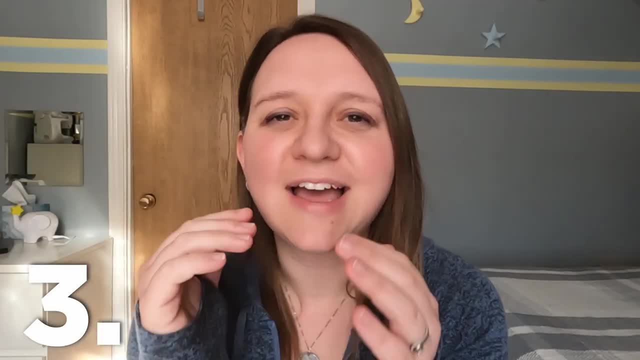 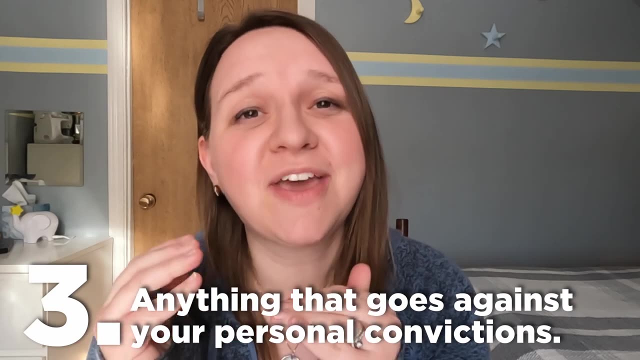 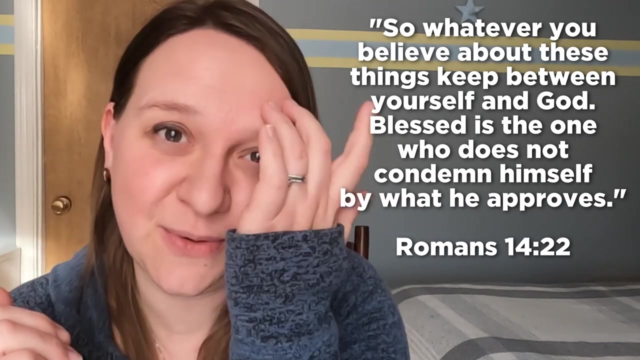 You should not purchase this year. Okay, While editing, I decided that I want to reword number three, which is: you should not use any curriculum that goes against your personal convictions. Cue Bible verse. So I have a story for you about this one. 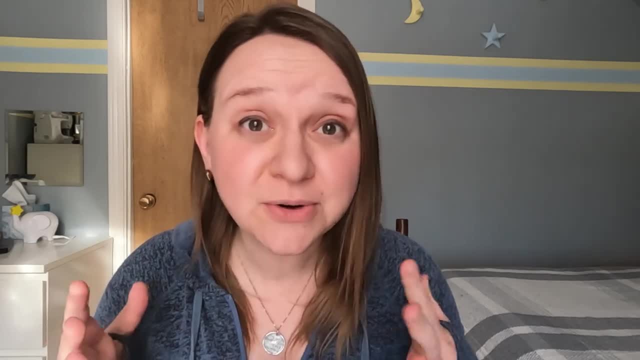 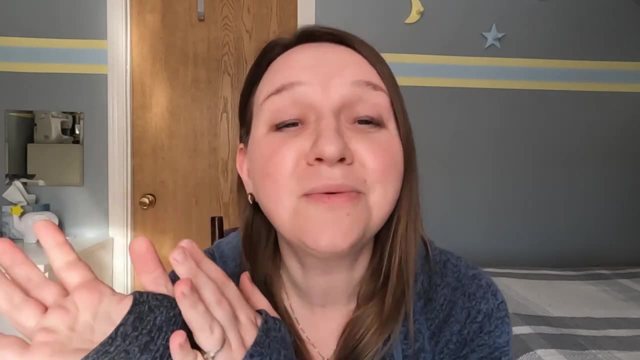 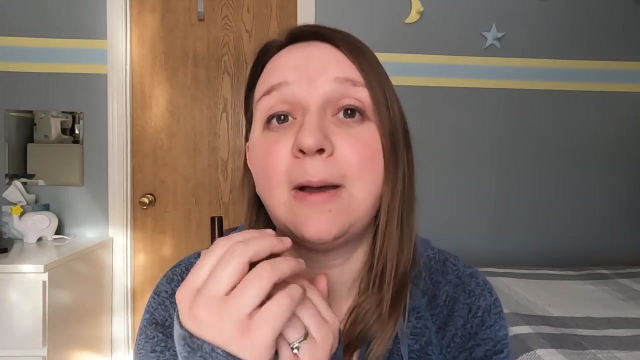 Last year I had a friend who actually bought a full curriculum for her kids. She has four kids and after they had already used it The year prior and been really happy with it. But now she heard something new about this curriculum and where it was coming from and started to feel: 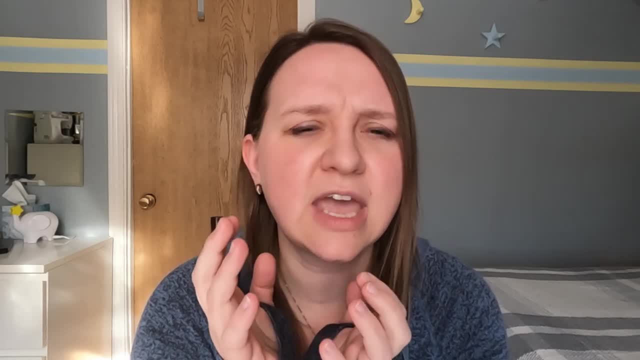 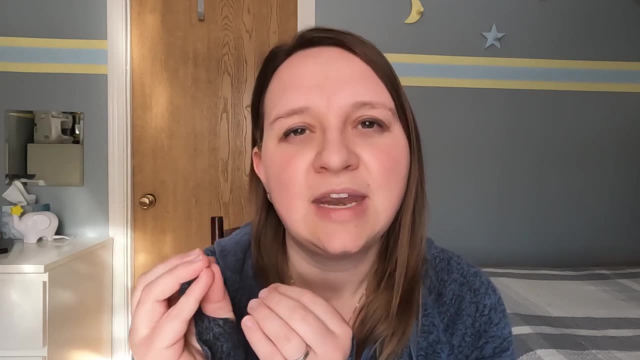 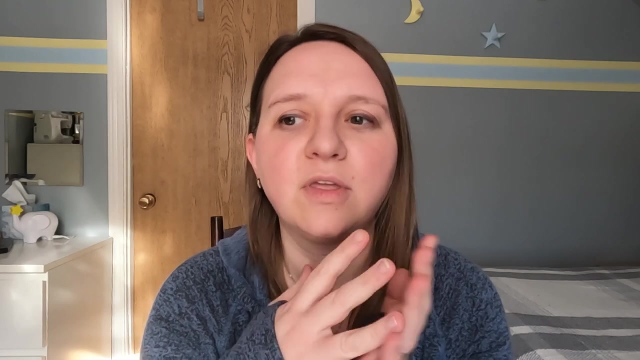 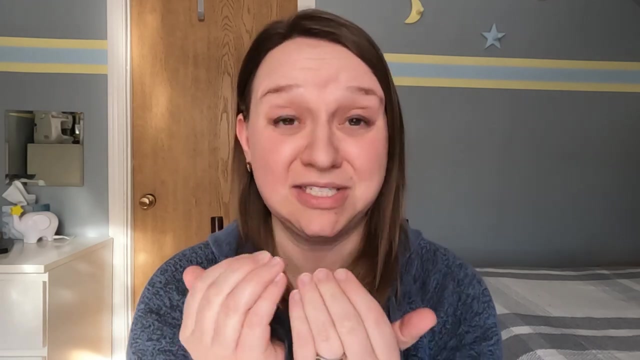 uneasy with it and then started to search and think and, and then she said things started to make sense, Like things that she had read and kind of questioned in her mind now made sense, understanding, um, the background Of the curriculum. And so she went to her husband and said I'm really sorry. 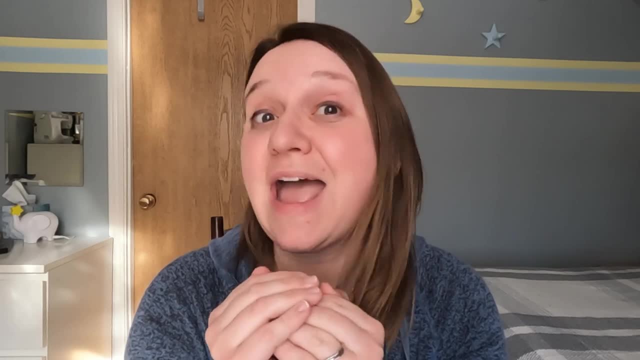 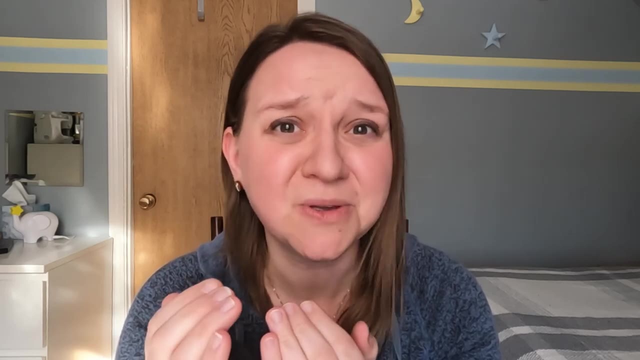 I spent money on this curriculum but I do not have peace about using it. And her husband instantly was just like you don't have peace about using it, Get rid of it. I don't want you using it with our kids. And so she did, she, she got rid of it. 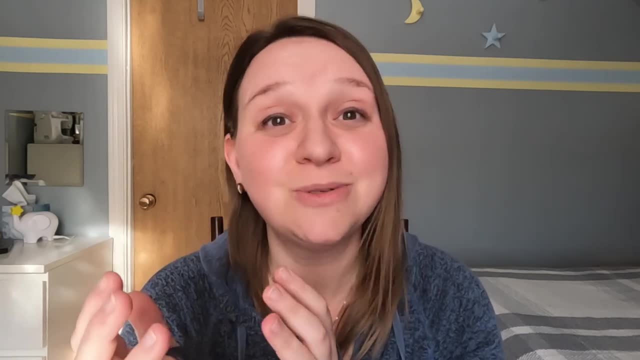 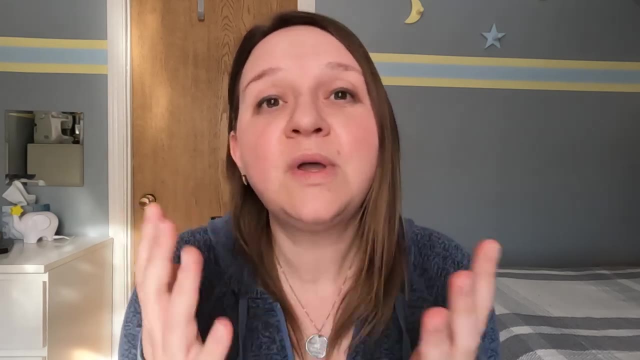 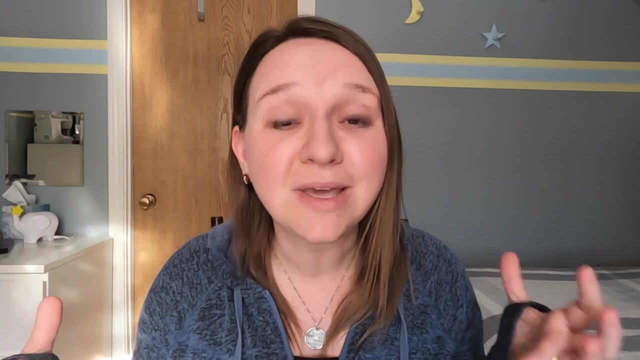 And last minute, when searching for something new to try it because she didn't have peace, she felt convicted About it. Now there, we will never know everything about curriculum, Probably it's. it's really hard to search through everything that we use, but if we are feeling convicted, 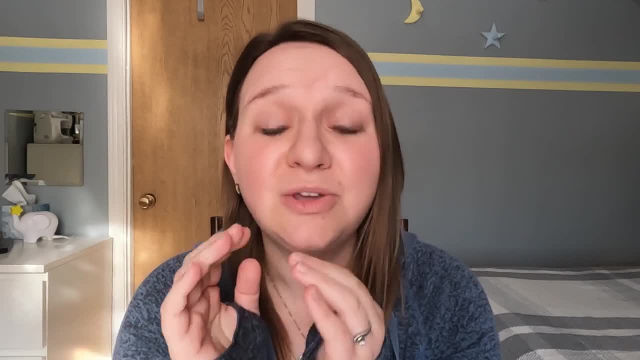 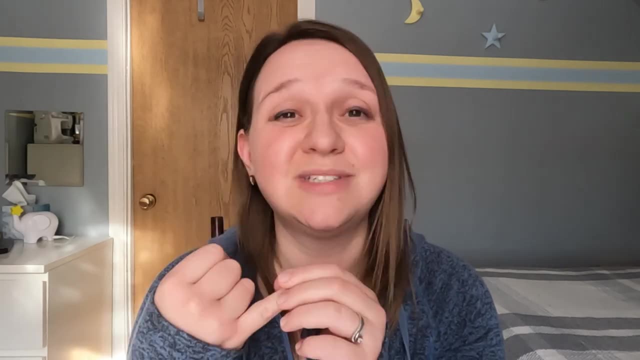 about something, we shouldn't use it, And you need to understand that you are an influencer Even if you don't have a YouTube or an Instagram. you are influencing your children. You are influencing your friends and homeschoolers that are observing. 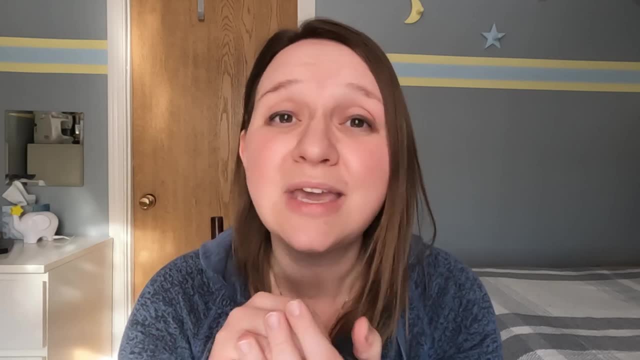 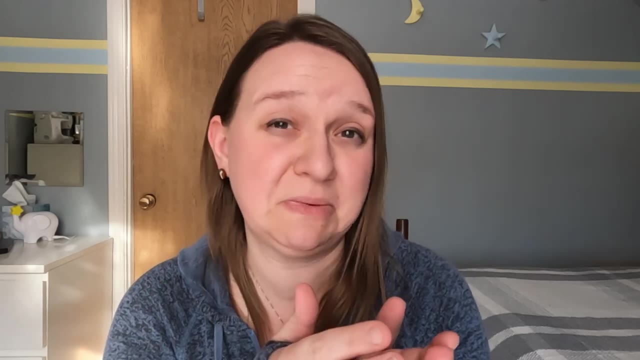 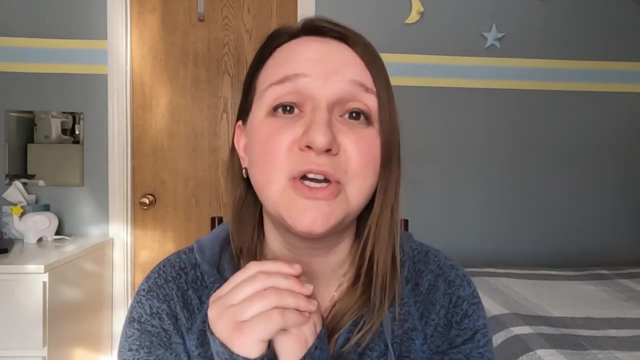 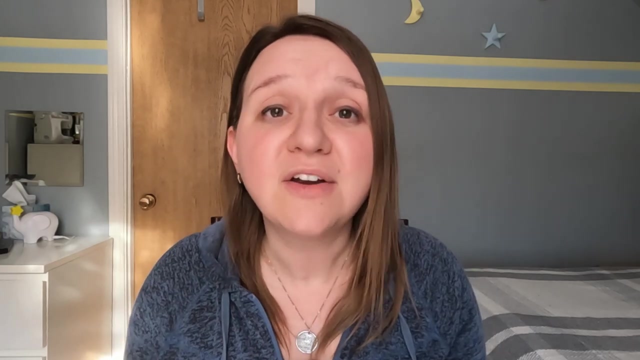 You, And if they see you using something and enjoying it, there is a high probability that they will want to try it out also. And while you have discernment, someone else might not, And we are to be very careful as Christians- especially if you're a Christian like we are to be very careful about what we are putting out there for others to see and use. 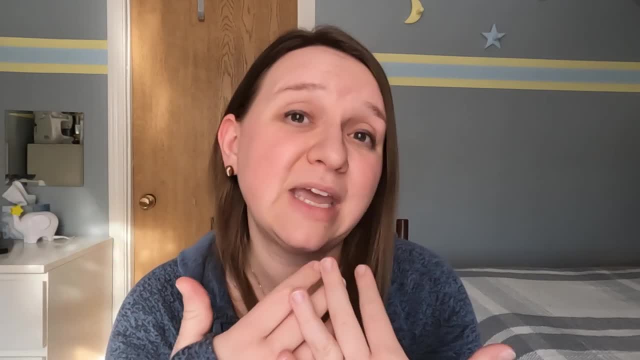 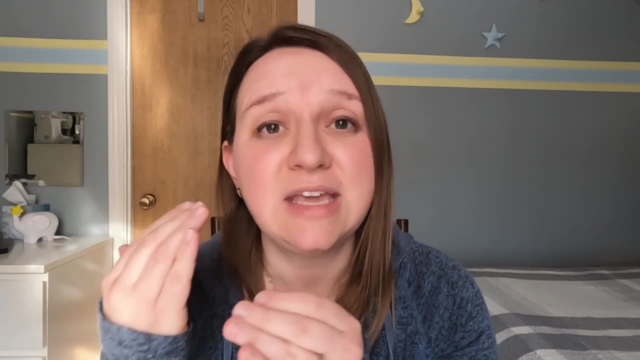 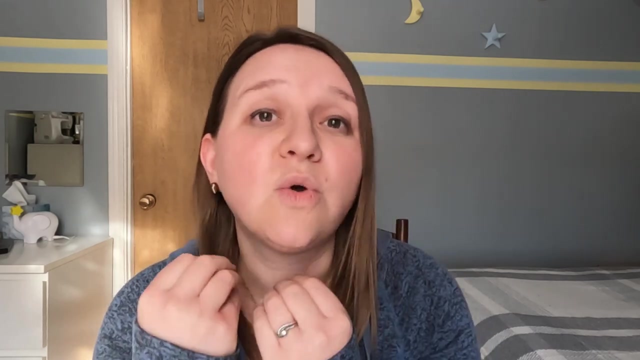 We are supposed to live so that others Can imitate us, And so I just want to reassure you. um, you should be looking into your curriculums and what you are using and making sure that you are fully at peace with what you use.